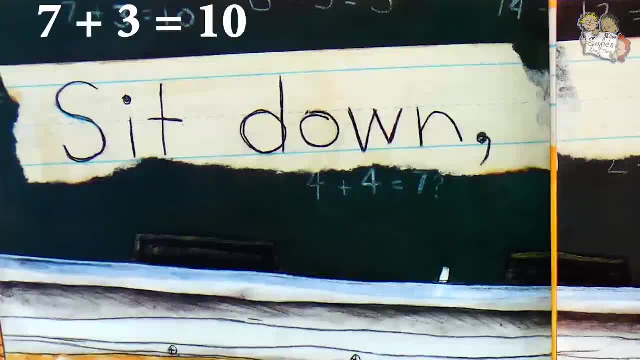 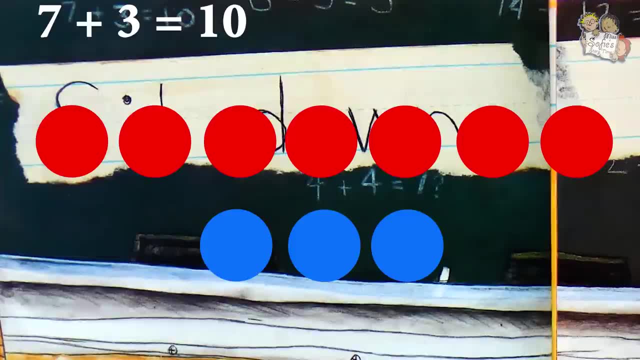 Seven plus three equals ten. That's correct. We have seven red circles and three blue circles. If we count them all together, it'll equal ten. Let's count them all together: One, two, three, four, five, six, seven, eight, nine, ten. 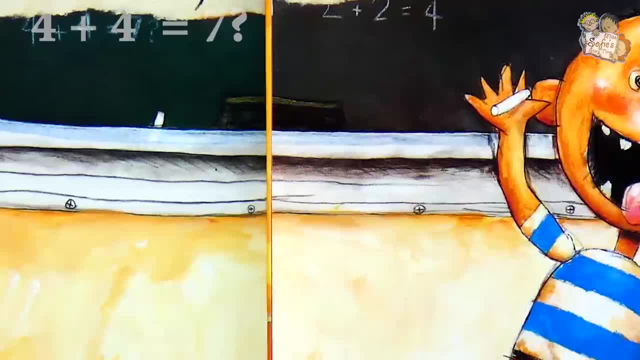 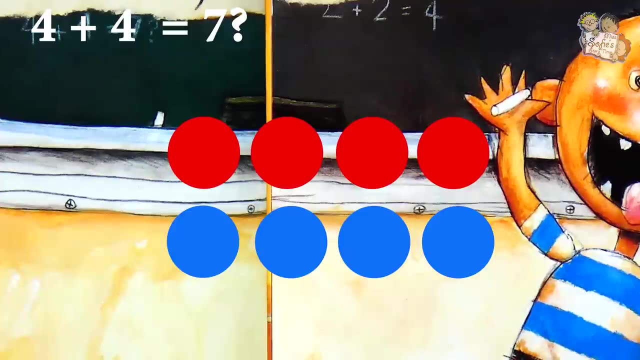 It's right. This one is: four plus four equals seven, But there's a question mark after it, so that must mean they're not sure. Let's double check it with circles again: Four red circles and four blue circles. Let's count them together. 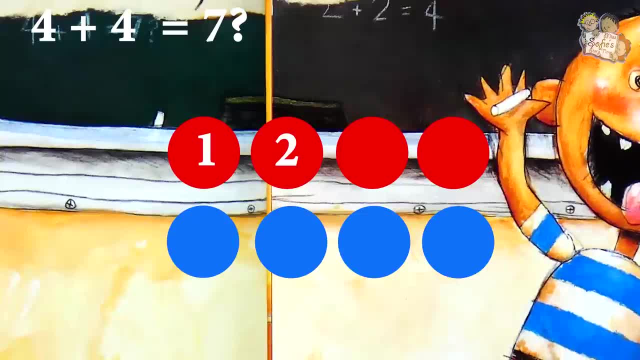 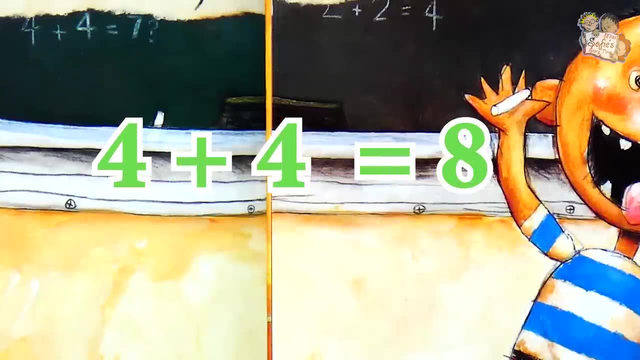 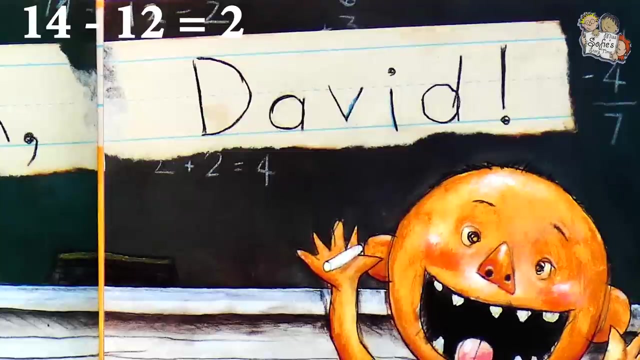 One, two, three, four, five, six, seven, eight, Eight. That one's wrong. Four plus four equals eight, not seven. Let's try the next one. Fourteen minus twelve equals two. Let's use the circles again. This time we're subtracting. 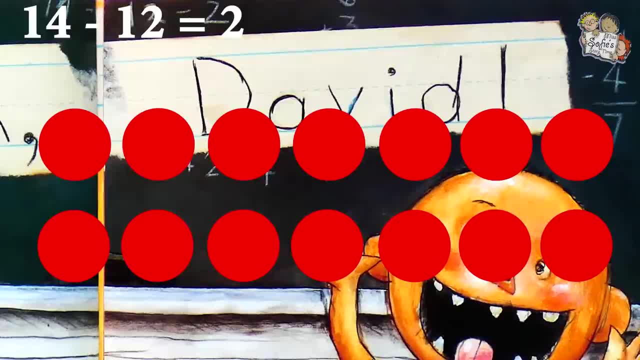 so we will take a total of fourteen red circles and count up to twelve and then see how many are left. Let's count together One, two, three, four, five, six, seven, eight, nine, ten, eleven, twelve. So now that we've taken away these twelve circles, how many are left? That's right. 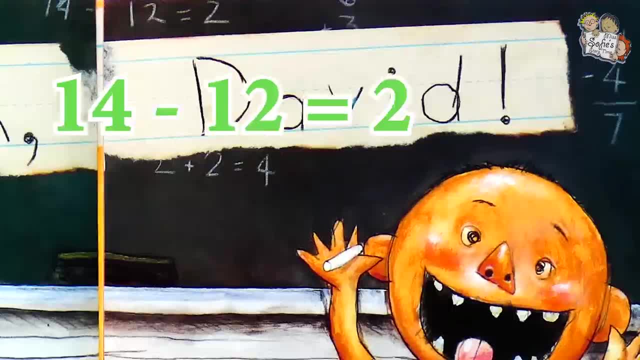 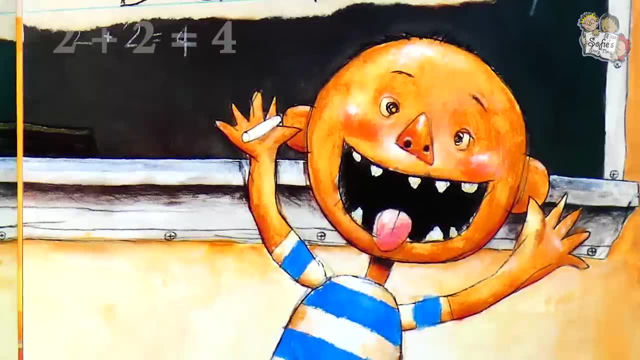 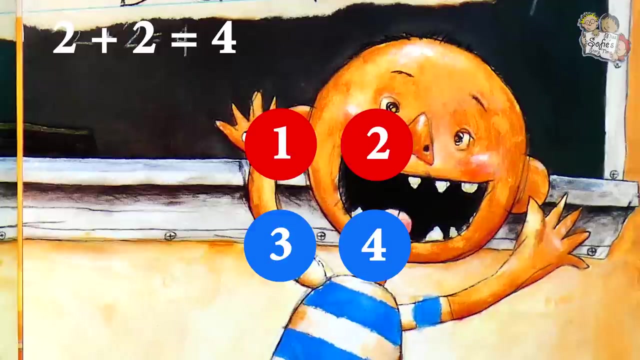 two. So fourteen minus twelve equals two. This one you might already know. without using the circles to count, Two plus two equals four. Let's try it one last time with the circles to double check: One, two, three, four. Yep, two plus two equals four. That one's correct. 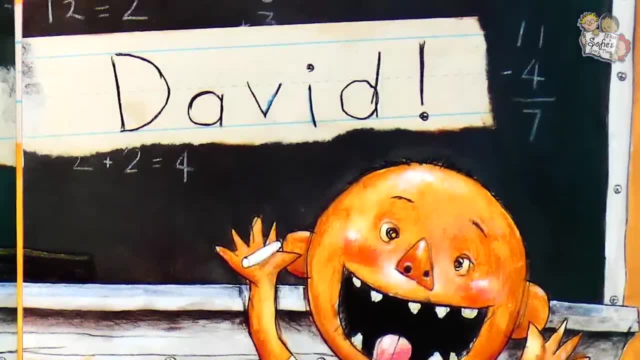 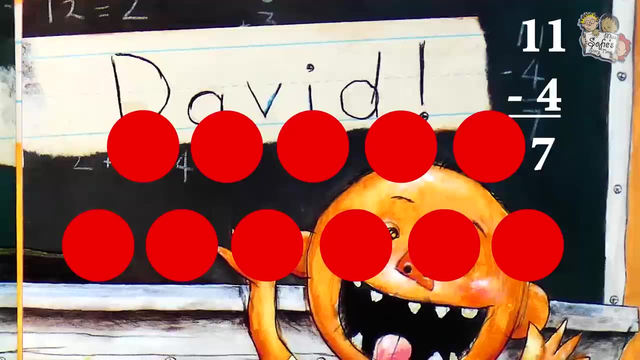 And the last one we can say here is: eleven minus four equals seven. This one is subtracting again. So we're taking away, So we start off with eleven red circles and we're going to take away only four of them: One, two. 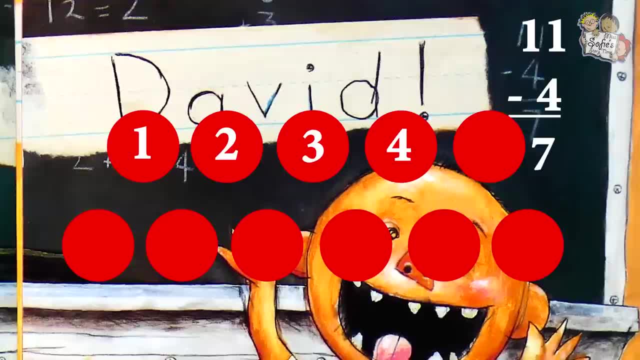 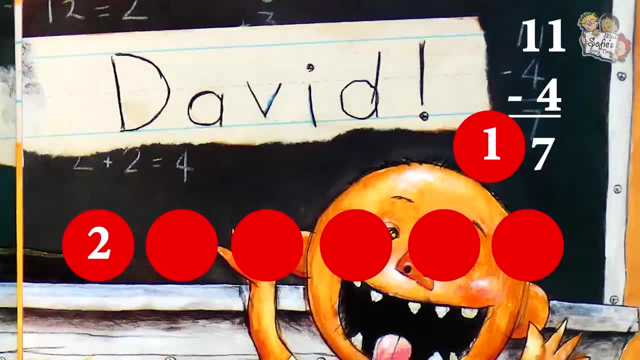 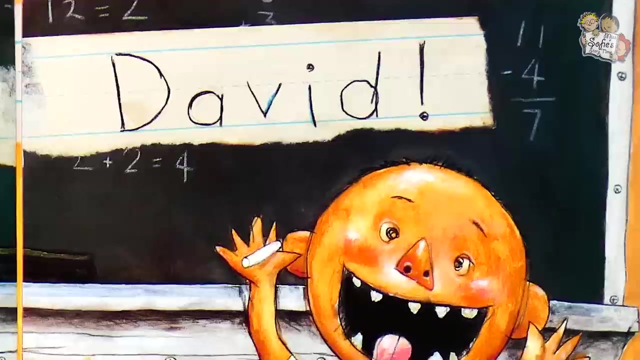 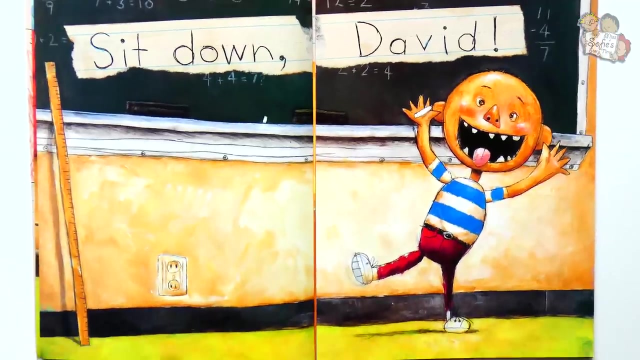 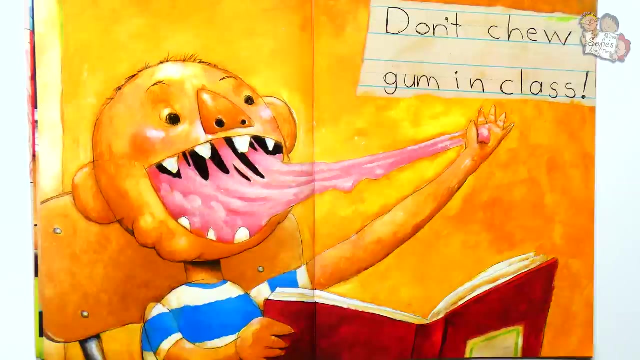 three, four. Let's see how many circles are left, and that will be our answer: One, two, three, four, five, six, seven. So eleven minus four is seven. That one is right too. So David only got one wrong. He must be learning a lot in school. Don't chew gum in class, Uh-oh. 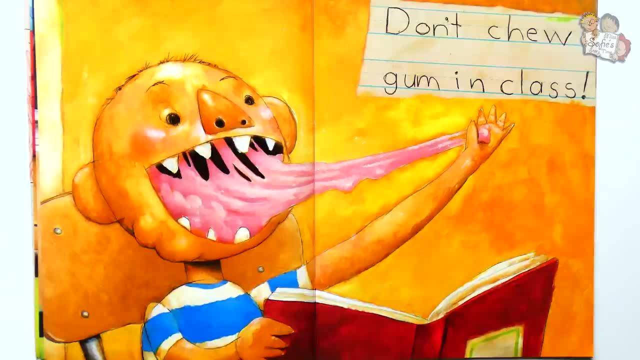 Chewing gum is not a good idea, So David got one wrong. He must be learning a lot in school, loud in schools. Have you ever stepped in gum by accident or found some stuck to your desk? It's so sticky and gross, Eww. 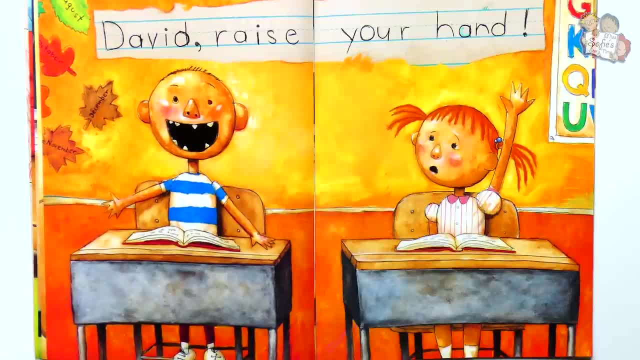 David, raise your hand. David is just shouting out answers, which means that other people who raise their hand patiently don't get a chance to answer the question. It's important to take turns. I wonder what kind of question he had to answer. The colorful leaves on the 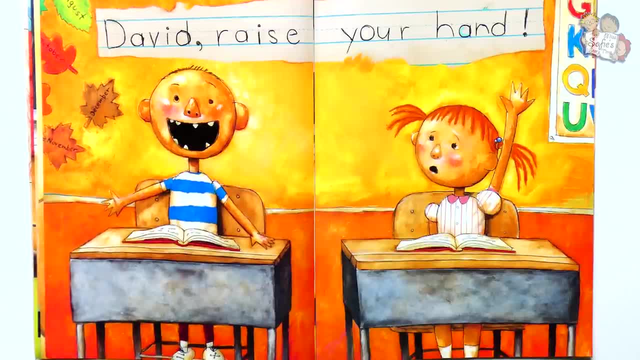 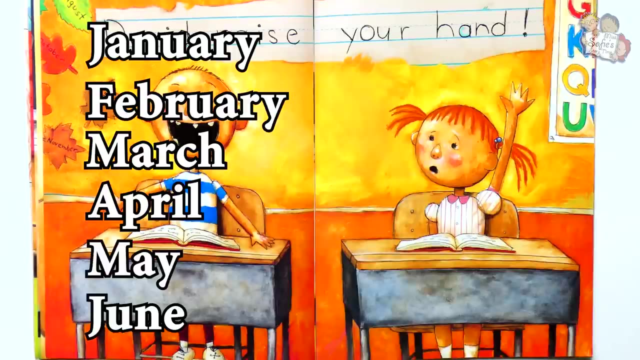 wall behind him are the months of the year. Do you know all the names for the 12 months? Let's list them: January, February, March, April, May, June, July, August, September. October May June, July, August, September. October May, June, July, August, September. 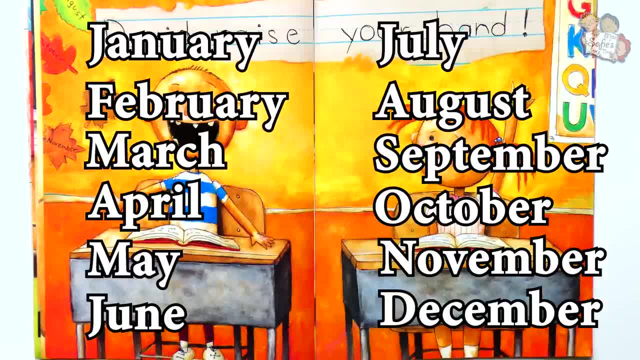 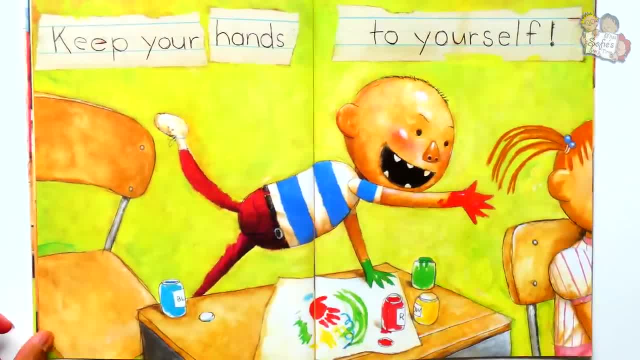 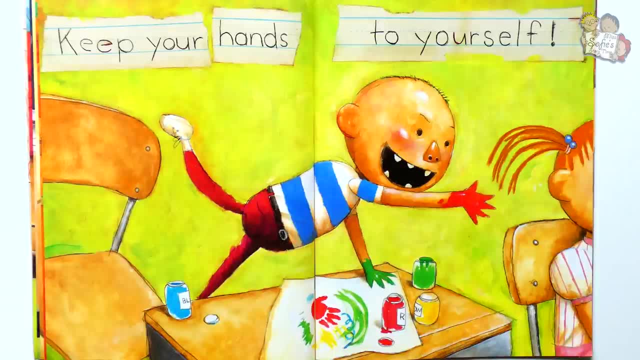 November, December. Great job, You're ready to go to school, just like David. Keep your hands to yourself. It sure is fun to finger paint, but if David touches anything else, he's going to get it everywhere On the desk and on his classmates. I hope it. 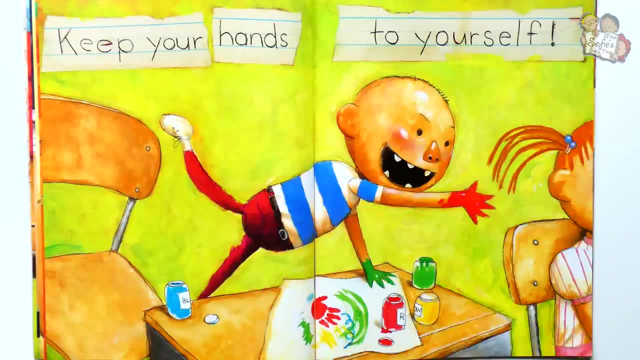 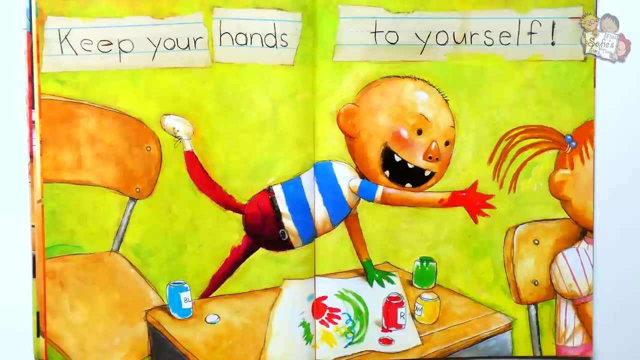 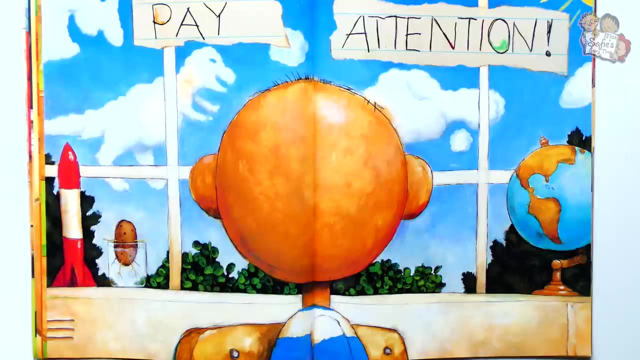 washes out easily. It looks like he's using four different colors. Let's see if he's using four different colors to paint with Blue, red, yellow and green. Pay attention, It's a nice day outside and it's easy to get distracted when sitting inside. It looks like David is. 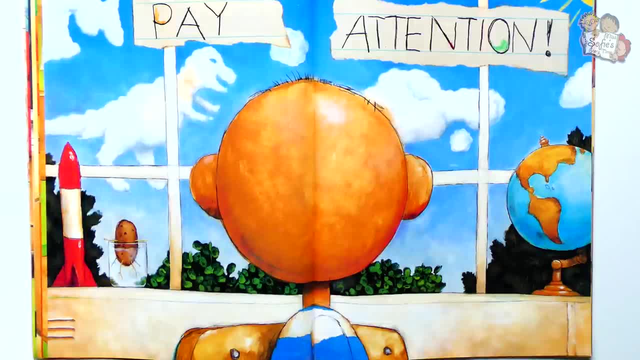 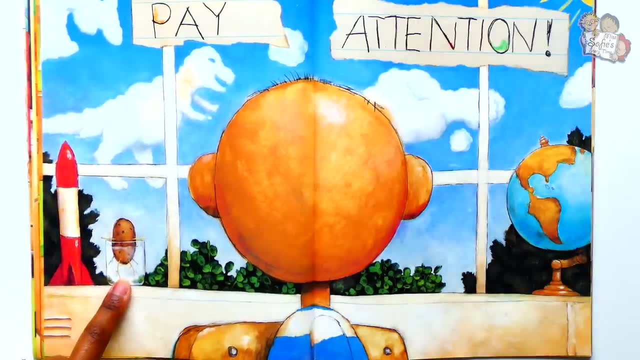 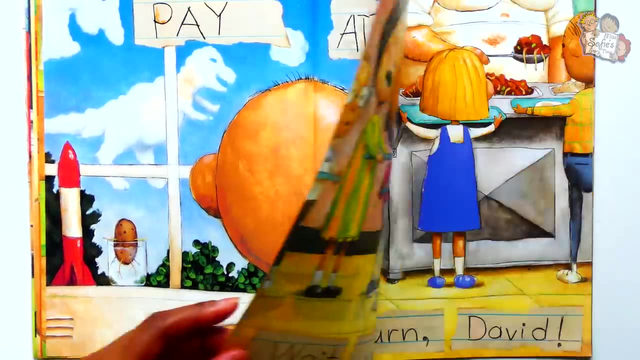 imagining dinosaur-shaped clouds instead of listening to the teacher On the windowsill. there is also a small rock. I'm going to throw in some rocks in the river. I'm going to small rocket ship, a potato growing roots in a glass of water and a globe. 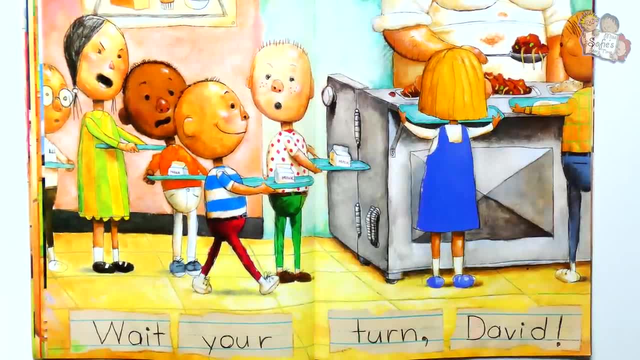 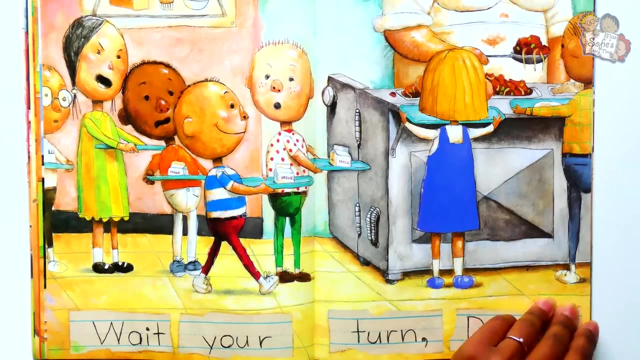 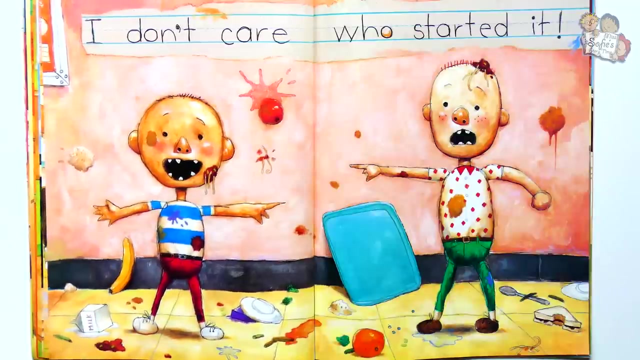 Wait your turn, David. David is cutting the line. I bet his classmates don't like that. He's supposed to wait in line like everyone else. They have milk already on their school lunch trays and are waiting to get food. I don't care who started it. 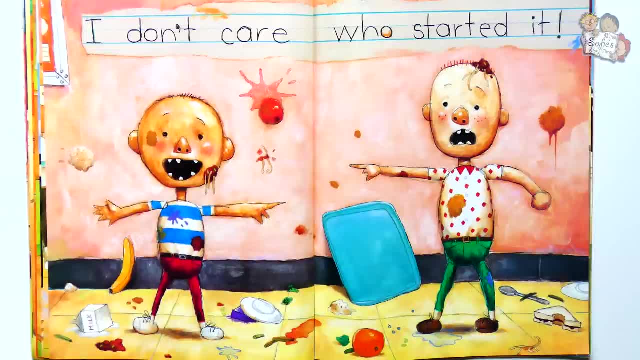 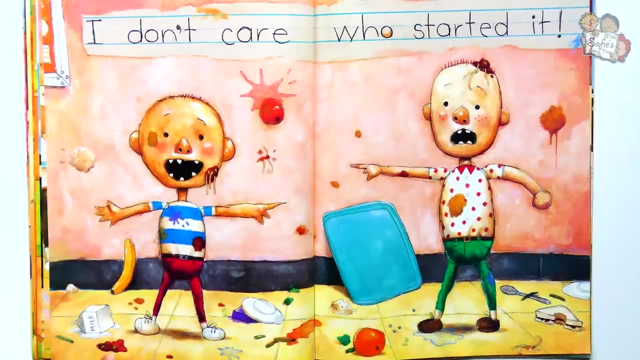 Having a food fight is not good. All of that good food has to go in the garbage now and their clothes are all dirty. It's not important who started it. It's about not making a mess and wasting food. They threw a banana, tomatoes, oranges and 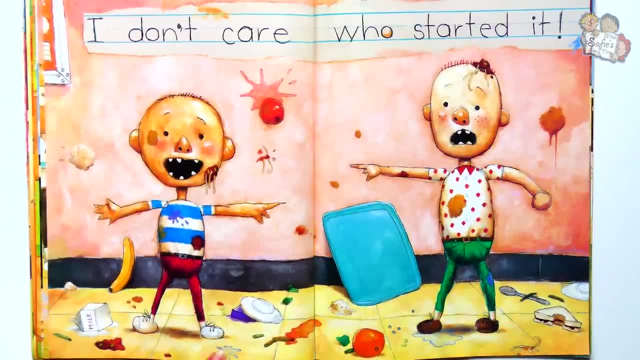 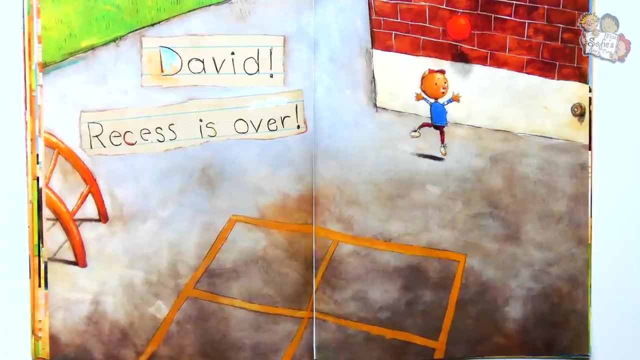 The milk, a sandwich and some other vegetables too. David, recess is over. It sure is fun to play outside in the middle of the day, but unfortunately David can't stay and play all day. Recess is only a short break after lunchtime. 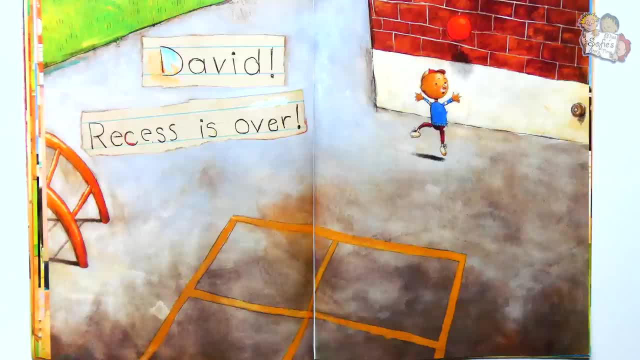 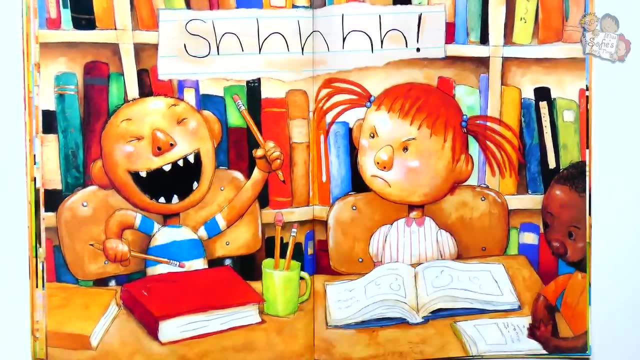 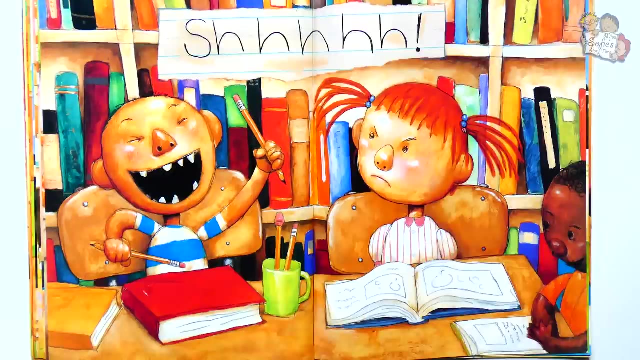 When it's over, he has to put the ball away and go back to the classroom and learn. David is being loud again, but do you know what kind of room he's sitting in? He's sitting at a group desk with his classmates and they all have books in front of them. 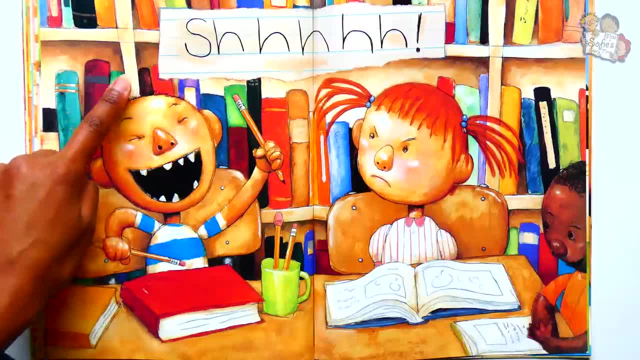 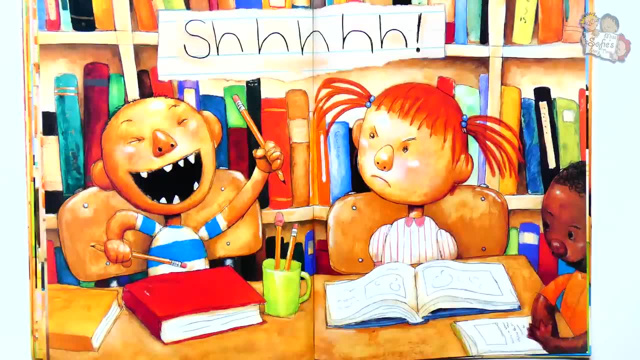 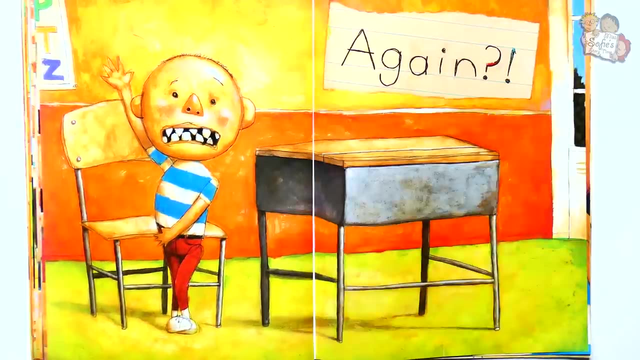 There are also bookshelves behind them with a lot of books on them. David is most likely sitting in the library, and in the library you have to be quiet. David has to go to the bathroom again. Sometimes it's hard to learn if you keep going to the bathroom during class. 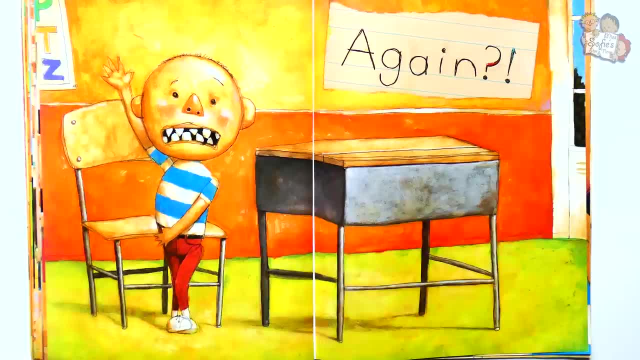 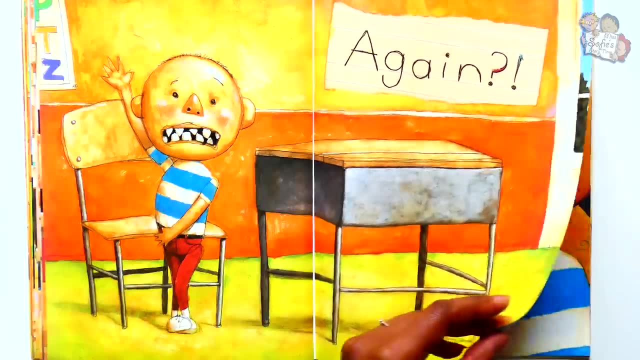 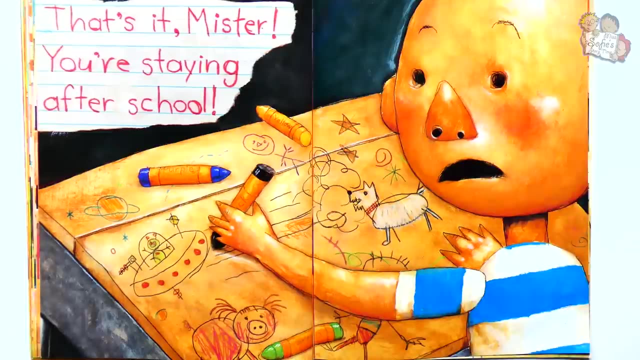 but if you drink a lot of water, which is a really healthy habit, then that's what happens. as long as he's not making it up to get out of class, That's it, mister. You're staying after school, Uh-oh. 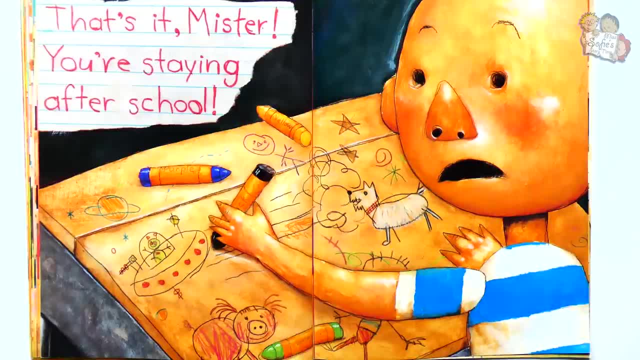 Now David is in trouble. Drawing on his desk is a big no-no. That's what paper is for. Other kids need to use the same desk after David goes to the next grade. I wonder what the teacher is going to have him do after school. 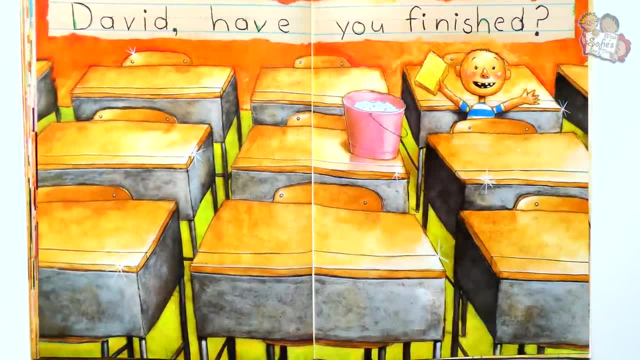 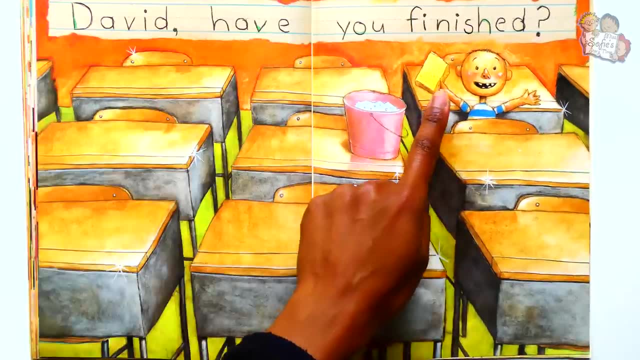 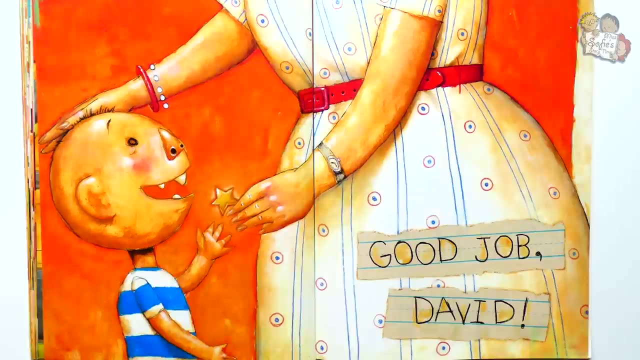 David, have you finished? David had to clean all the desks, but now they are nice and squeaky clean. He used soapy water and a yellow sponge to clean them. Good job, David. David's teacher is giving him a gold star since he cleaned all the desks so well. 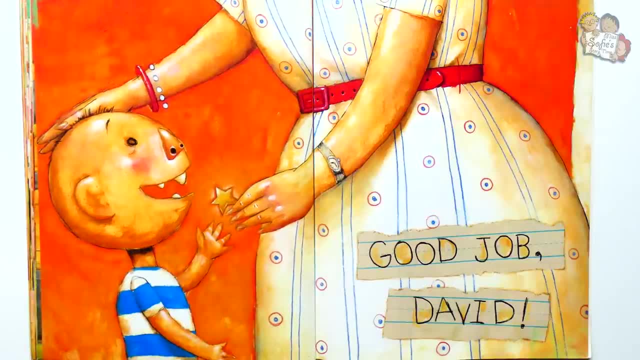 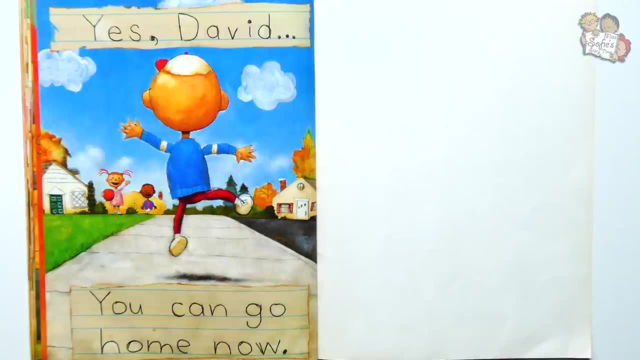 He cleaned not only the desk that he drew on, but all of them. Yes, David, you can go home now. After a long day at school, David is finally finished. He's happy to go home and play with his friends. The end. 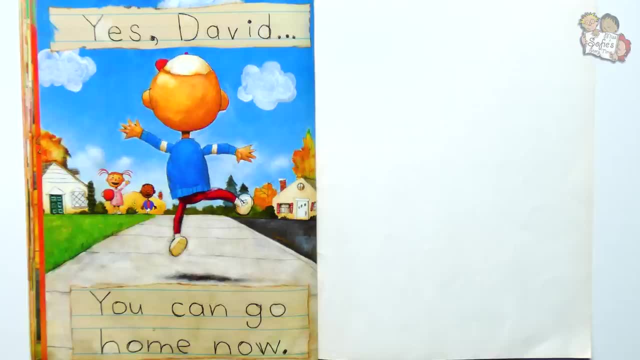 David is learning every day about what to do and what not to do in school. When things are new, sometimes you're unsure about what to do, But there will always be an adult, like a teacher or your parents, to help guide you. So be sure to listen to them and learn from them, just like David. 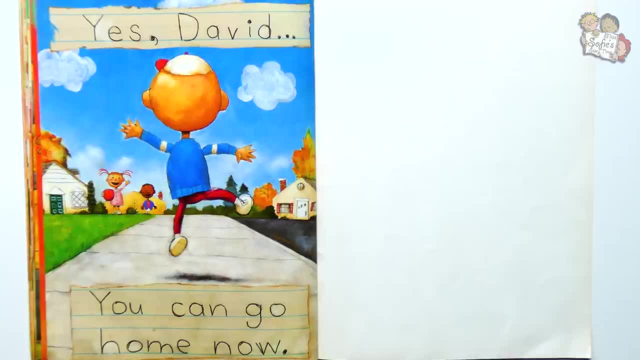 To read other books, subscribe to our YouTube channel. Subscribe to this channel by clicking on the red subscribe button. This way, you can always find this channel and listen to more stories. Keep reading, and until next time I'm Miss Sophie's Storytime.